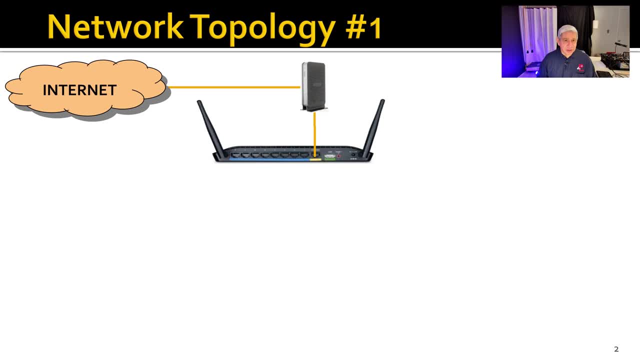 the internet service provider, or it could be one that you bought, like I've done. I think I'm now up to my fourth one. for this particular configuration, It's given an outside address. Now, this is an address assigned by the internet service provider, which you have very little control over. You have 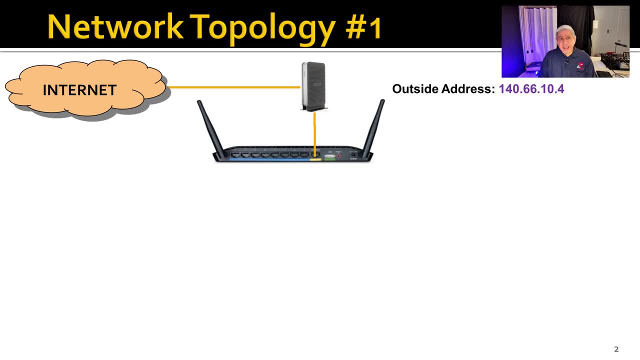 to know how they've set it up. So you have to configure certain parameters in the router in order to get it set properly, but you have no choice in what the number is going to be. That's what I'm going to do, So I'm going to go ahead and set it up. So I'm going to go ahead and set it up. 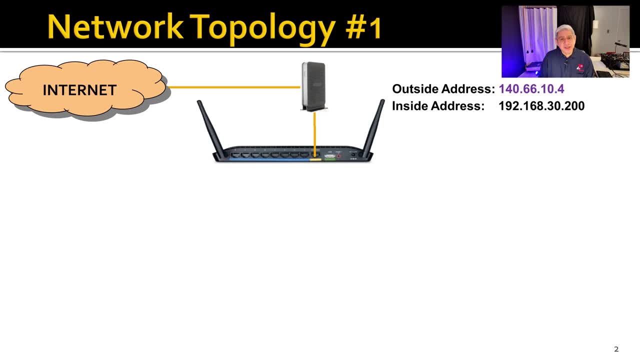 for the ISP on the internet. but you can assign the inside addresses, And what I've assigned to this particular router is 192.168.30.200.. And you'll see how that's derived in a few minutes. I've also chosen a subnet mask. The subnet mask of 255.255.255.0 means that we have a total address. 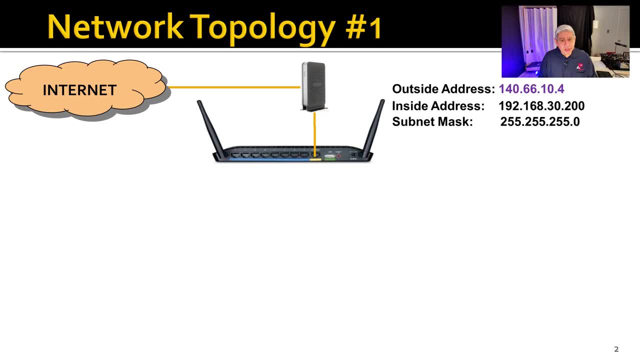 space that includes 256 addresses, amongst which 254 are usable, as I'll explain in a little bit, And you can set up the address space directly through hard wire. That's what I'm illustrating here, with the blue lines up to your router. In this case, I have two desktop computers and I 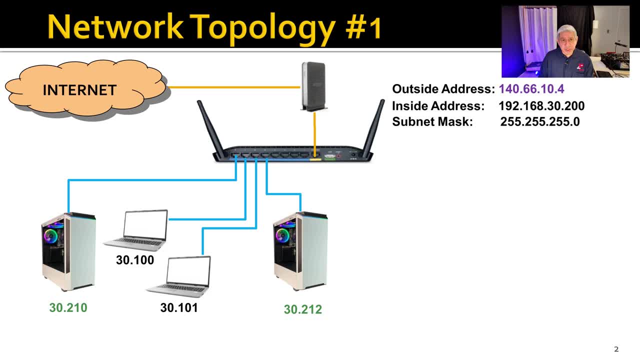 have two laptop computers and they are hard wired up to that particular router. Now I'll get into what the addresses mean in a moment, but those are also within an address range that I've selected. In this case. we also have a lot of wireless devices. It could be an all-in-one computer. 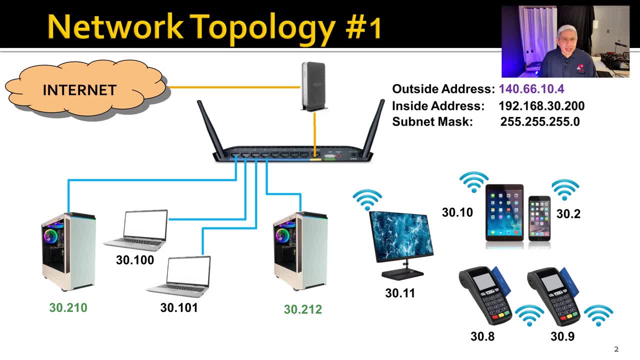 It could be iPads, It could be phones, It could be anything like that. I have down in the bottom there actually point of sale terminals, for example, if you're a small company. Now the address has come out of a range, as I said, which we pick, and I'll show you how to pick that later. 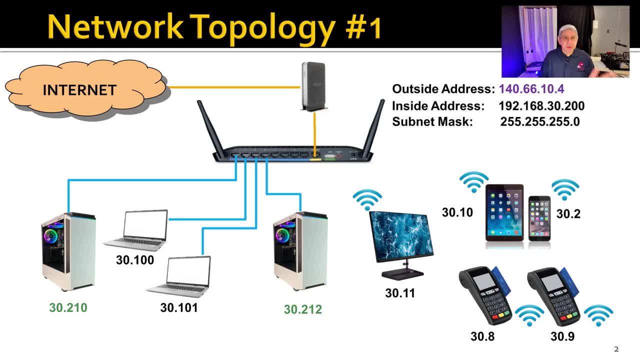 when we set up the actual router, because you can define what the minimum and maximum address range within your allowable addresses of 254, which ones of those will be automatically assigned by your router when something is connected. Point to note here, though: two of these are not automatically. 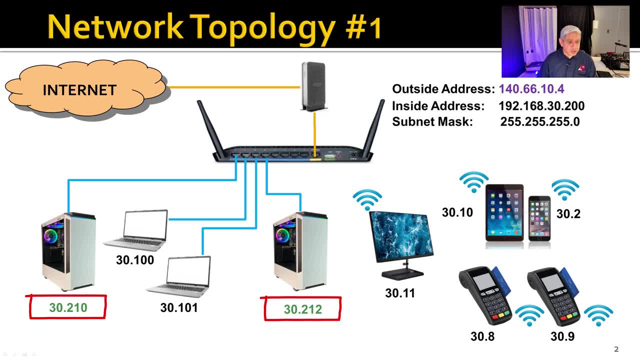 assigned, The ones I have in green, the two workstations, the two towers here. those have been statically assigned in the router And I'll show you how that's done when I go into configuring the router in a few minutes. All the rest were picked through the DHCP, a special service that's. 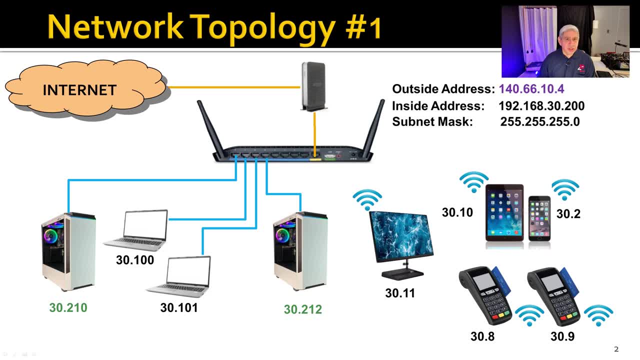 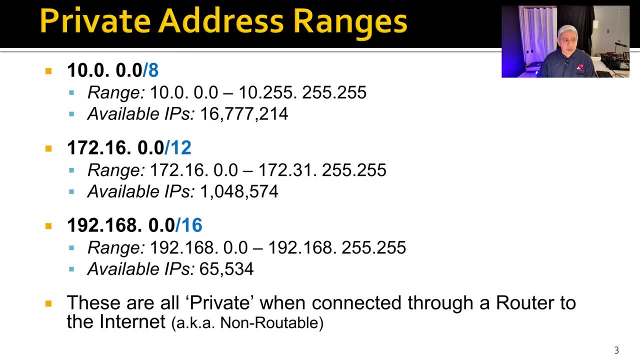 running on your router that will dish out addresses that are requested by a newly connected device. Now let's look at private address ranges. There are three of them. I talked about them in a lot of detail in a previous video, so I'm not going to get too involved here, But generally the one. 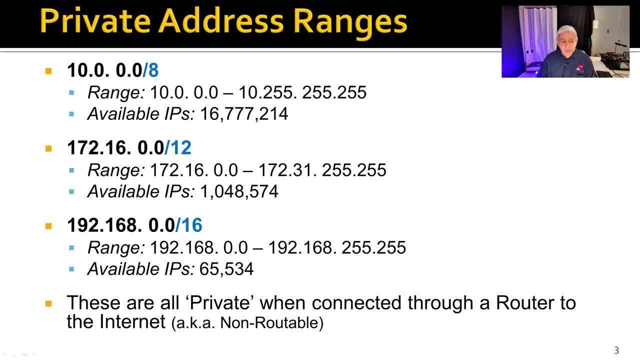 that we call it 192.168.0.0,. that particular address range is the most common one. that comes on routers you buy for a home or a small office, Pre-configured. there's an address range in it when you first turn it on. That's usually in that range, The middle one, the 172.16,. 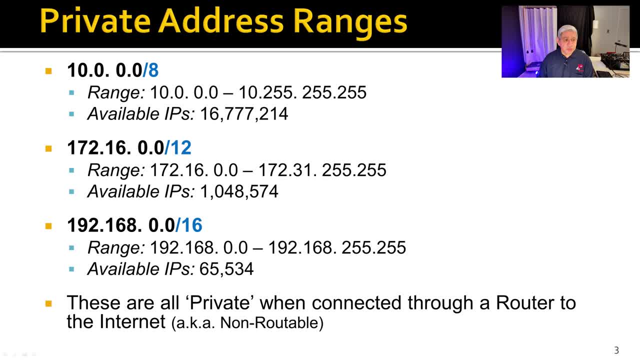 that's usually for slightly larger organizations, because it gives you more addresses, Whereas the 192.16 range gives you only 65,000. and change: the 172.16 range gives you over a million And if you're a really large organization you would use the 10 dot. 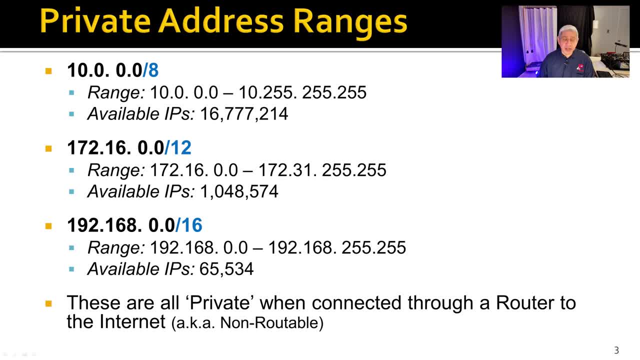 and that would give you over 16 million addresses. You get to choose any of these you want when you go to assign your network addresses, But you know usually people stick to the 192, or, like I like to do, you go into the 172 category. It's sort of a little more secure because that's not one that's. 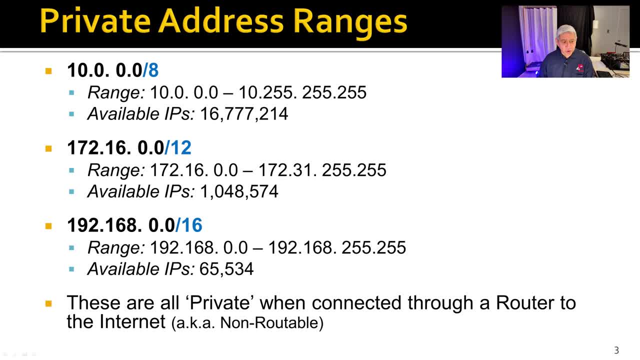 expected by someone that's trying to get into your network And, as I said before, all of these are private, which means it will not pass through your router to the internet. The router will make a conversion, A network address translation, or NAT, which will change your internal addresses to something that. 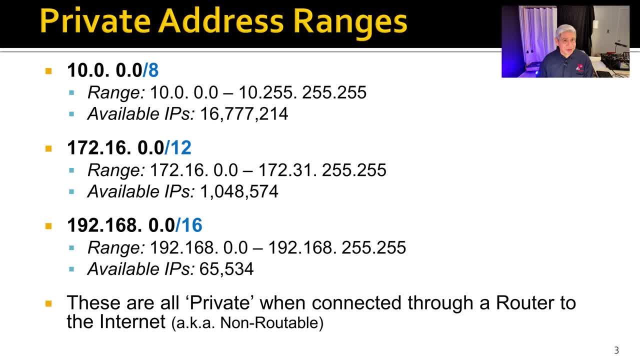 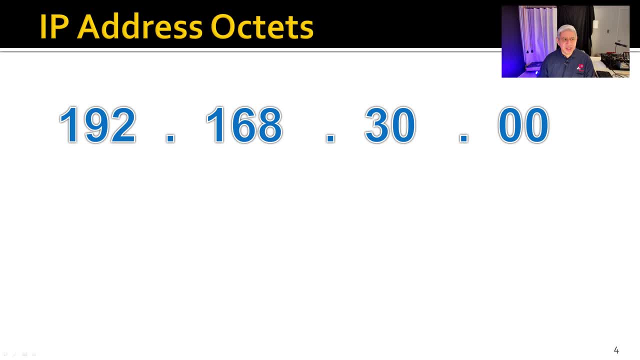 looks like the outside address, the one provided by your ISP, So just keep that in mind. It's getting a little bit in the weeds, but it's an important concept to understand as we start to configure this. Now let's break this down a little bit more. The four different numbers here are: 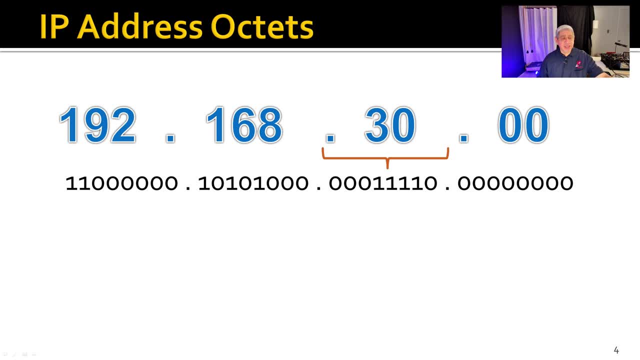 called octets, and they're called that way because they have eight bits of binary, which is octal, right Eight is oct, And since there's four of them, each one has eight bits, a total of 32 across the board. Then each one of these is one octet, or one quarter of that 32.. 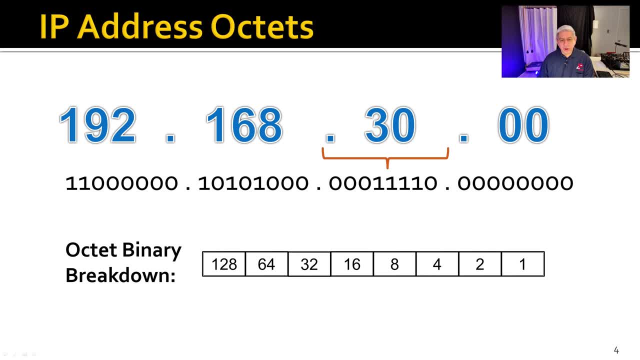 Now that's defined, each one of these, by the binary table. So all the way to the right is the weight of one. So the zero in all these cases over here, if it were set, has a value of one. The bit all the way to the left, which a couple of them are set: the 192 has it set and the 168. 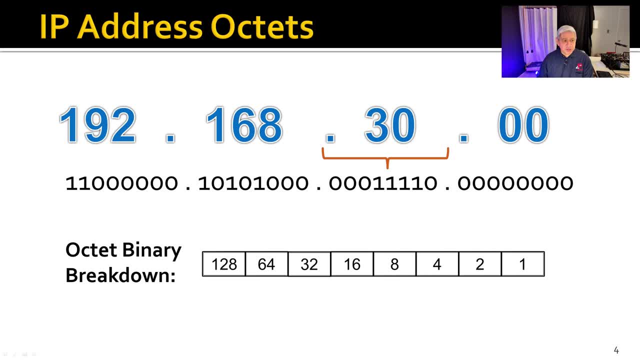 has it set. that represents a value of 128.. Whichever bits are set, you just count those numbers up and that will equal the address. Or you could use a calculator that converts decimal to binary, Or you could just go on the internet and say: how much is 168 in binary? 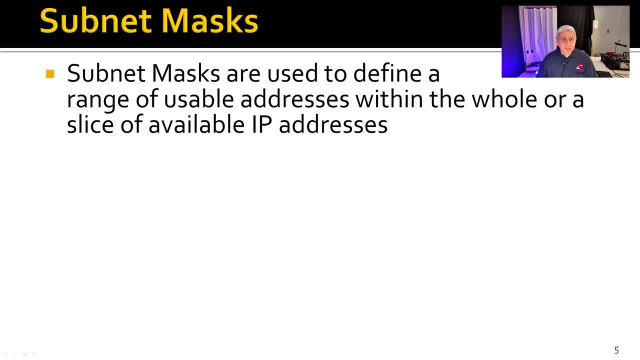 and it'll give you those eight bits. Now let's talk about the subnet mask. Now, this is sort of a little bit convoluted explanation, but I'll go into a little more detail. It is used to define your range of usable addresses. That's the bottom line to it, And you 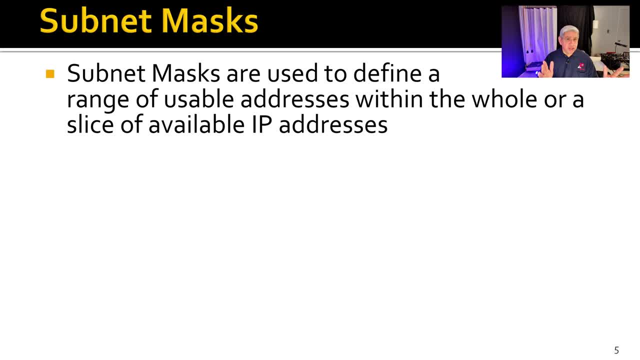 can define your range of usable addresses as the whole chunk that you initially wanted it to or, as I mentioned in my other more detailed video, you could break it into smaller networks, but I'm not to cover that in this video. The most common subnet mask for small businesses and homes is: 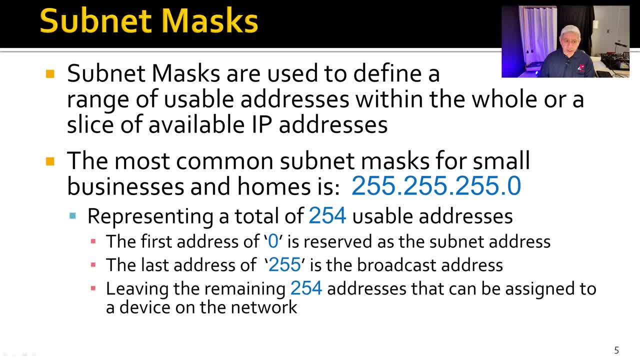 255-255-2550, like I said earlier, and that gives you 254 usable addresses. since the first one, the zero is used to represent the actual subnet address. So when you're asked for a subnet address, you always end it with that zero at the end. in the case of this particular subnet mask, If you 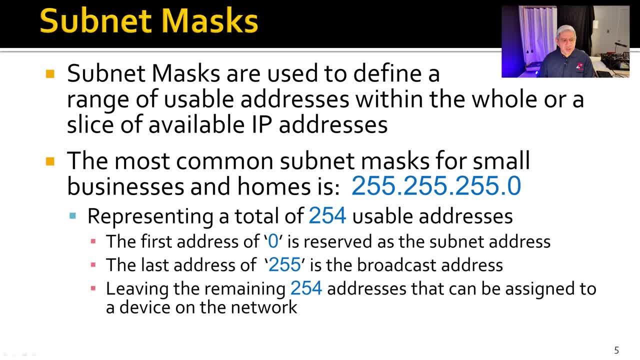 want to do a broadcast to every device on this network. that's what the 255 is for. So if a message is sent to any address network and the network address in our case would be 192.168.30, and then we put 255 at the end, that same message will go to every device on your network. You don't? 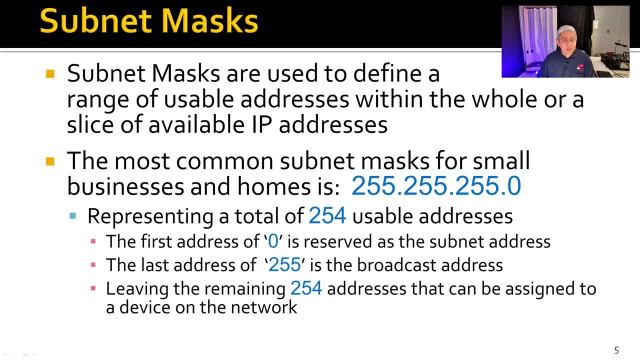 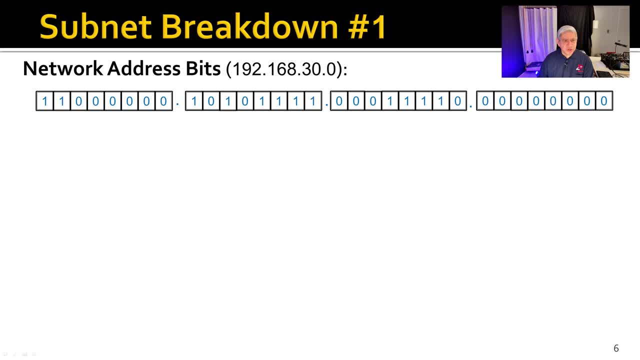 normally do that, but the devices that you connect to it might, So just keep that in mind We have. that's why it's a reserved address range in most cases. Let's look at this and breaking it down a little bit. We saw this earlier. This is the actual network address that I chose and we broke it into. 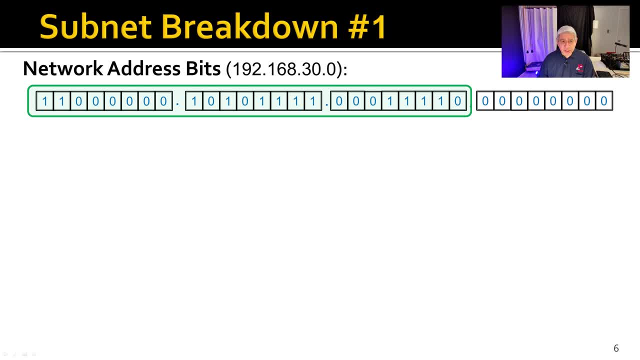 its four octets in binary. When you look at this, though, the one that's in the middle is the one that's in the middle, So if you're looking at this the way it works, the first 24 bits represent the network address. The last eight bits represent 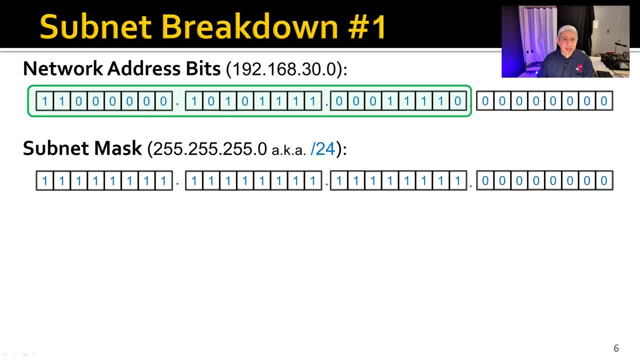 the device address, and that's determined by your subnet mask, as I described earlier. And it's done that way because 255, 255, 255, zero, it sets all ones to the left, The first 24 bits and the ones that are left zero, all the way to the right. Well, they become what's left over for your addresses. 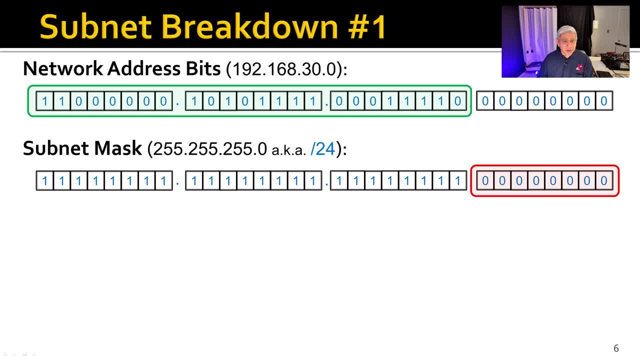 for your devices that are on that network. So part of it is your network and the remaining part of it is your device address. The network part is fixed. It'll always be that number. It does not change. This is also referred to as a slash 24 because when you convert this 255, 255, 255, zero. 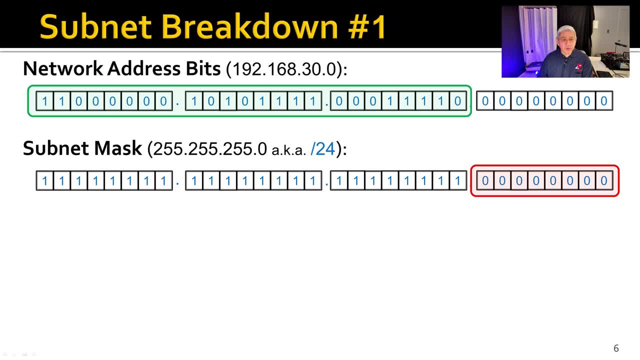 into its octets and binary, you have 24 bits that represent the address. So a shorthand notation. as I explained in another video in a lot more detail, it's calling it a slash 24.. The actual address range you then have by picking this, assuming that the only thing that's going to 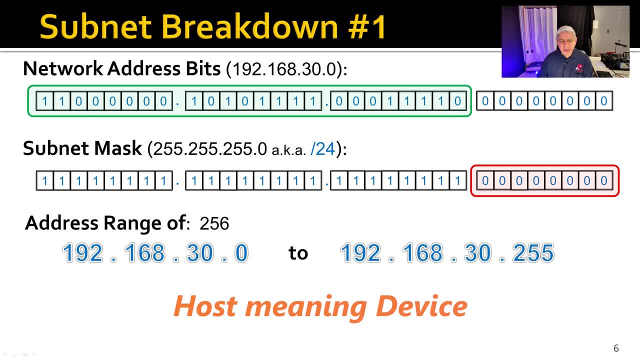 change. here is the host address part, the last eight bits. Then it'll start off at 192 168 30.0.. That's the lowest address in the range up to 192 168 30.255, which is the broadcast address. The 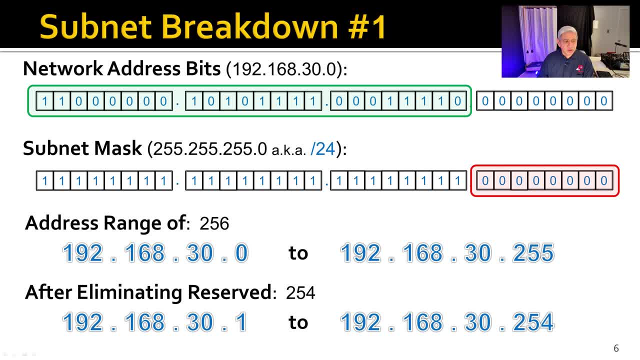 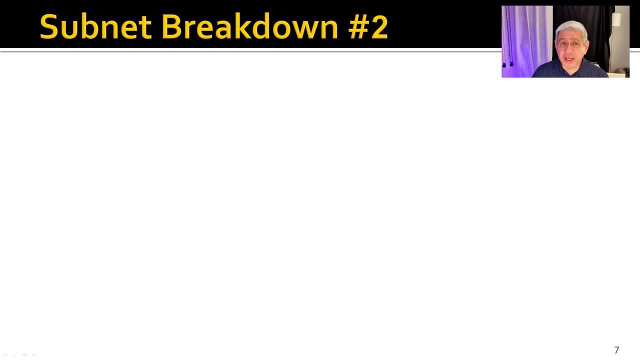 two ends are not usable, but all the ones in the middle are, So this gives you the actual usable address range when you've defined it. So it starts off at 30.1 and goes up to 30.254.. I'm leaving that for simplification purposes. What I want to show you, though, is a second alternative subnet. 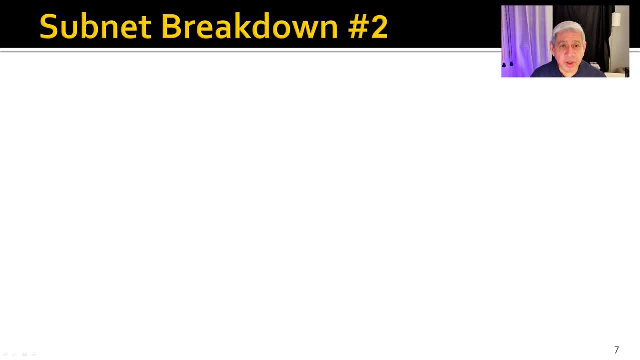 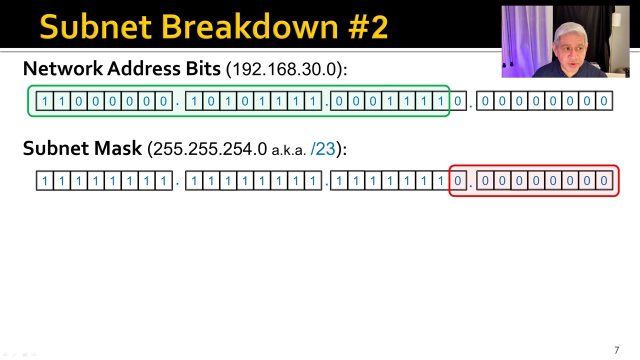 breakdown and this is the one I'm most likely going to use. In this one, we actually have the same network address of 192.168.30.. However, and that would represent the address, I'm changing the subnet mask to 255, 255, 254.. And what that does for you. if you look at what I have now highlighted, 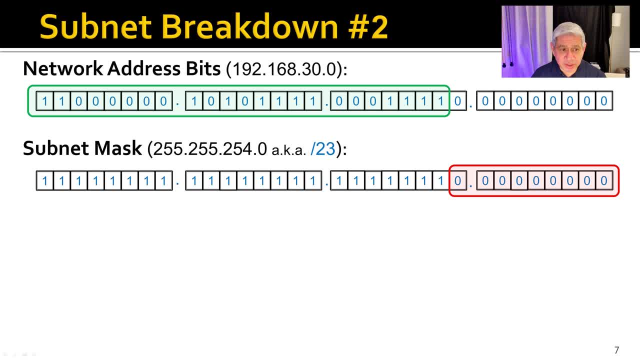 in green and red is we only have 23 bits for the address, because I have 254. that last bit in that octet is not one, it's zero, as shown here in the subnet mask. By doing that it rearranges the address part and the device address part. So now we have 23 bits but we have 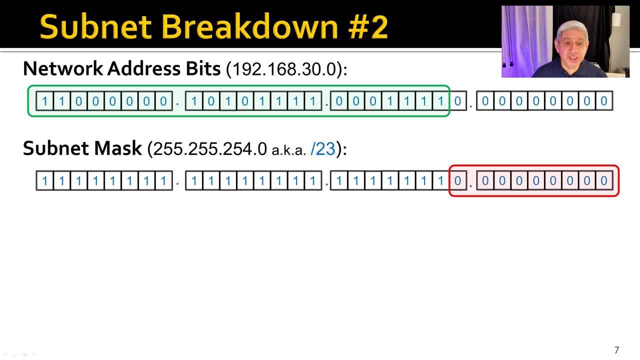 nine bits for the actual devices. What that'll do is double addresses for devices rather than having 256.. We now have 512.. Again, though, minus the two, it comes out to 510, which is, you know, more than double the actual address. So that's the last bit, and that octet is not one, it's zero, as shown here. 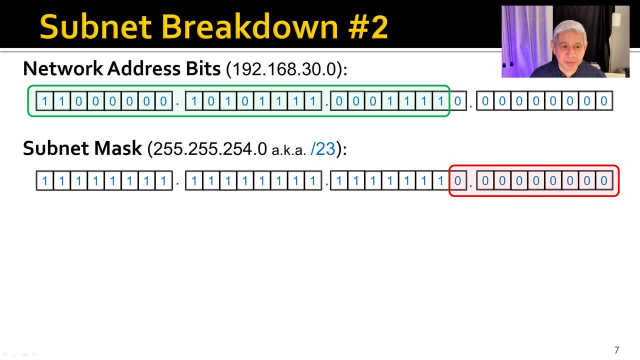 in the address space that I had before. with that one little change of the subnet mask and the new range of all addresses is 512, with the lowest being the dot zero but 30.0 and the highest being dot 31.255.. Now we set that extra one bit there, because now that one's in play. So if that one 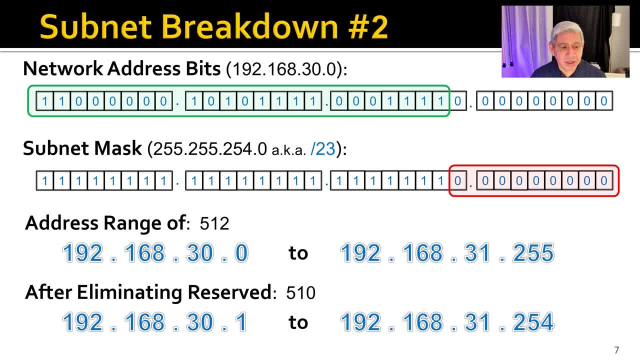 gets set, it covers the other half of that, 512.. Again, subtract the two, we have 510, which will then result in a total usable address range from 30.1 up to 31.254.. And if you add that range up it's kind of hard to do the math. it's not normal math. 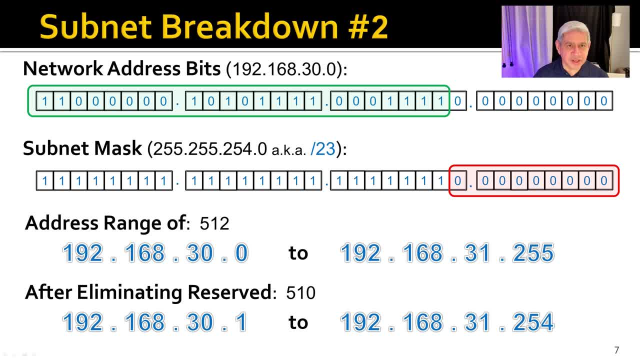 here. The fact that we set one automatically gives you 256, and then we add to it another 254, that comes out to 510 addresses. So this is important to understand: just by changing that one bit, how it changes things around. I could take this even further, but now we've got to be. 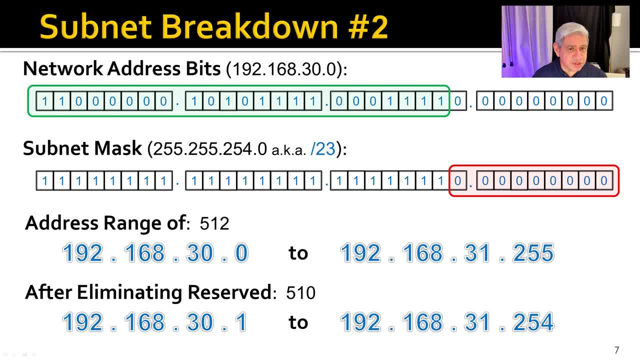 careful, because the address is actually using some of these other bits. If I wanted to make it say 10, 1024 addresses, I would have had to pick a different address than 30 so that this bit would not have been needed. So I could have made it 28.28 would have worked fine rather than 30. And that. 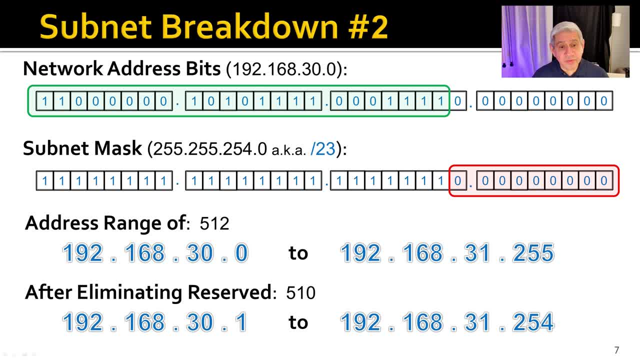 means that this bit would have been cleared for the address, and then I could have used it for more devices as one example. This is the tough part of this, and you'll see in practice, as I set it up on the particular router a little bit later. Now, one thing I do want to cover is, in addition to setting 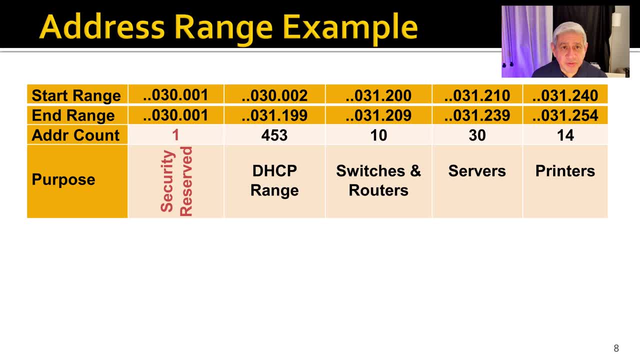 addresses in a particular group which is much larger, in this case 510 addresses. I want to reserve certain groups of those addresses and that's what I'm showing here. I'm going to do something very specific Now. a lot of this is just documentation, and then I have to follow through in. 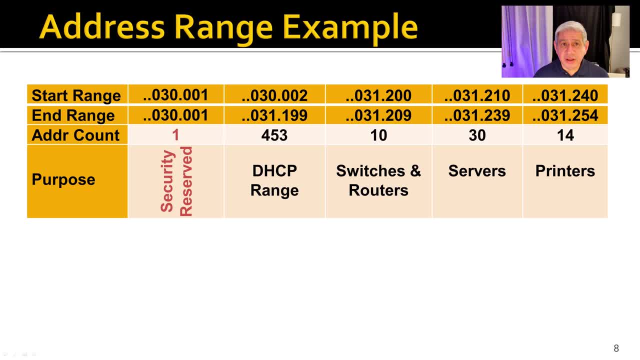 that documentation when I configure the addresses on the devices and I configure the router. The only part that I really have to tell the router about, though, out of this, is what is my DHCP address range, and I'm going to tell it. this is again based on the previous example. I'm going to tell: 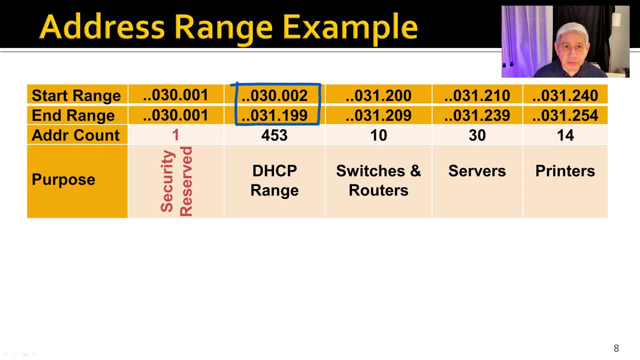 it that my DHCP address range will start at 030.002. that's the lowest address that can be given out. Of course it still has the 192.168, but then it'll be .30.2. that'll be the low one and the highest. 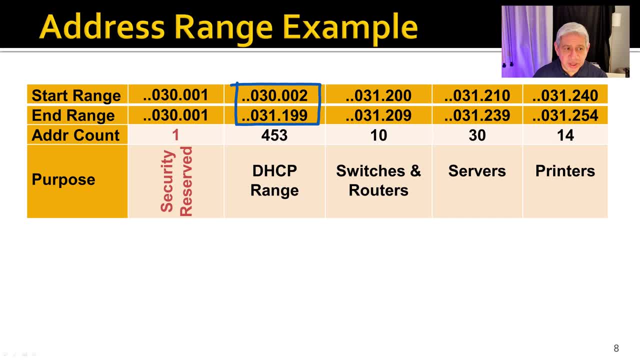 will be .31.199.. That'll come out. if you did the funny math, then you get 453 addresses available for your DHCP ranges. That's a lot more devices that are available to me for DHCP. but a lot of devices are indicated on the initial address range. So I'm going to tell it that my DHCP address range 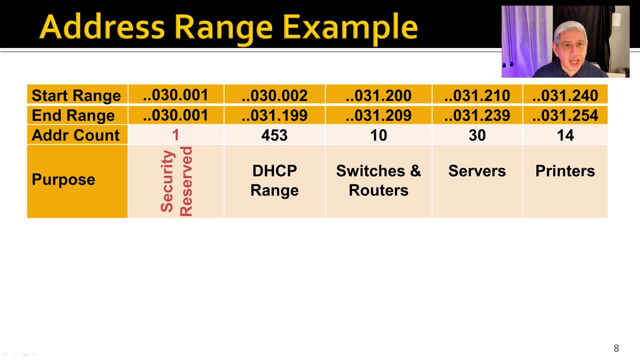 for example. I am not going to use DHCP for those. I'm going to hard code them, I'm going to make them static addresses and I've chosen groups of addresses for doing that. So starting at .200 or .31.200 and going up to .31.209.. There's 10 addresses in that range. That's where I'm going. 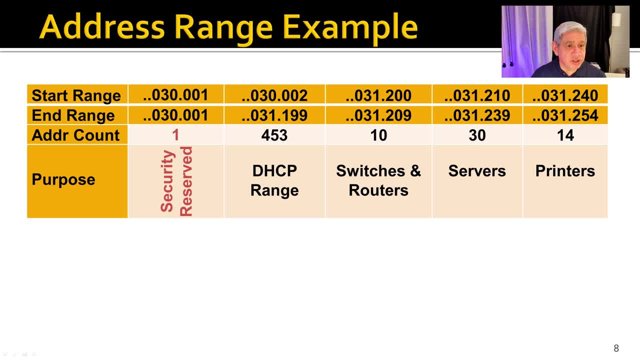 to put my switches and my routers. I have more than one, so I'm going to assign those addresses in that range to those devices. They're not going to be drawn from DHCP. I'm going to do it static. for my servers I set up a range of .210 to .239, or a total of 30 addresses. Those are going to be. 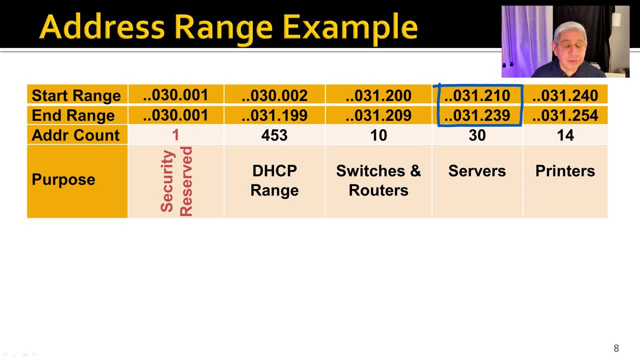 my servers that I have in my network. I don't have that many now, but someday I may, and I'm going to do the same thing for printers. I actually have two printers right now, but I'm reserving space for up to 14.. Will I ever use it? Probably not, but this gives me some flexibility. I know now. 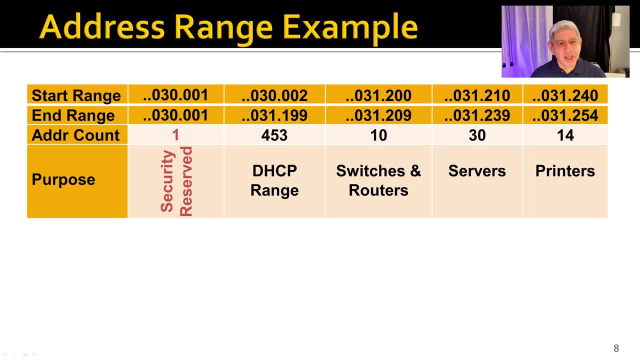 that I'm organized in a way where I always know where to look for printers, I always know where to look for servers, I always know where to look for the switches and the routers and the DHCP. The DHCP will then have this range to dish out to any device that doesn't have a static address. 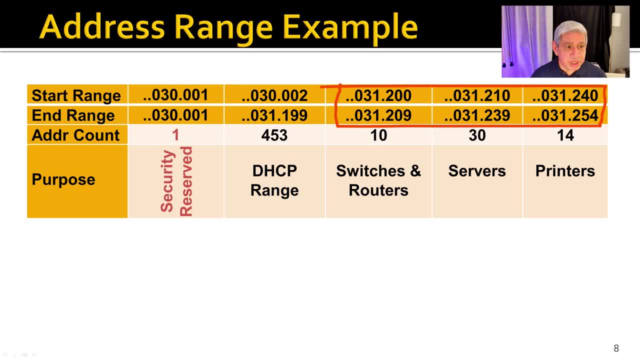 assigned to it. It will not touch any of these addresses because they're outside of this address. that I will tell the router. What I've also done is I've reserved the very first address that would have been usable, the .001, the 30.001 to be specific. I'm leaving that unused. Now there's. 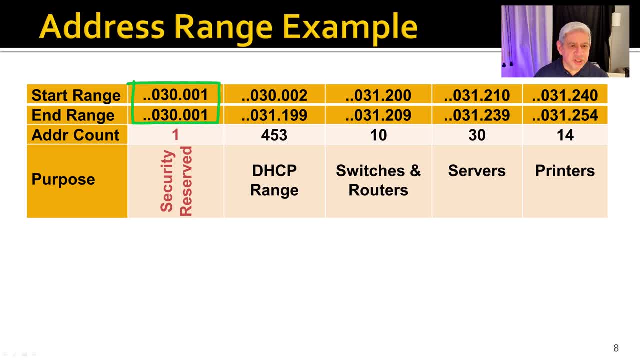 a reason I'm doing that. That's for security purposes. That's why I put my switches, including my router itself, up in this address range, starting at 200.. I don't want somebody, if they somehow get some information about my network, to look at the first address, because 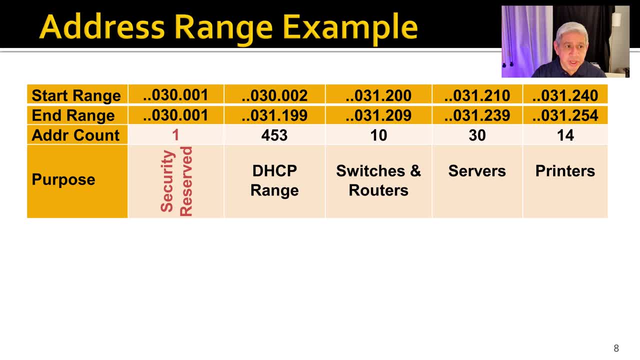 if everybody does it and the routers themselves of default to it. If you pick a network address of, like I did in this case, 30.000- then it puts the router at one. Well, you can change that, It doesn't have to be at one. So I am going to put it at a high address so that it's not obvious It. 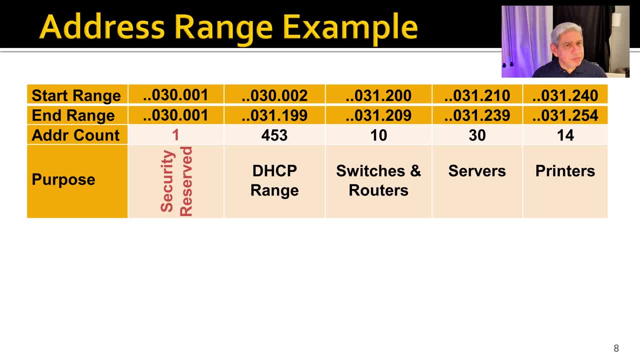 makes it a little more difficult for somebody to try to understand my network and then hack into it. It's just a personal choice based upon the fact that I'm a security person by heart and by meaning as well, early on in my career. So, anyway, this table. here is how I'm doing it You could do. 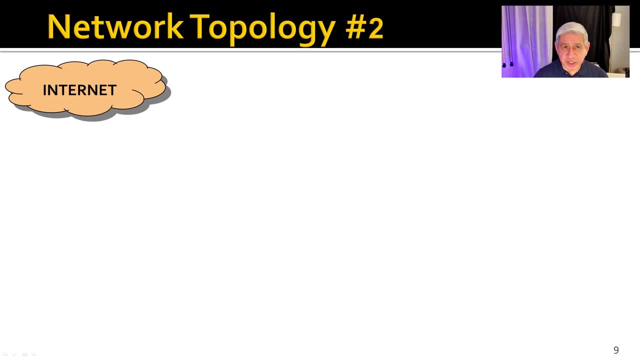 it a million different ways. Now let's look at the new topology that this will cause. I'm calling it topology number two. We have the same thing: The internet cloud. We have the modem, We have the router. We have the same outside address. We have the same address, with one difference for the actual 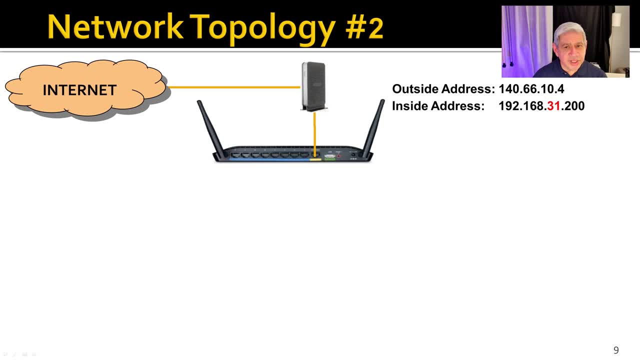 router. It is no longer .30.200 but .31.200.. I'm pushing it into the upper 256 addresses that I have available. What's up on that table? I just showed you The subnet mask and I've highlighted in red the 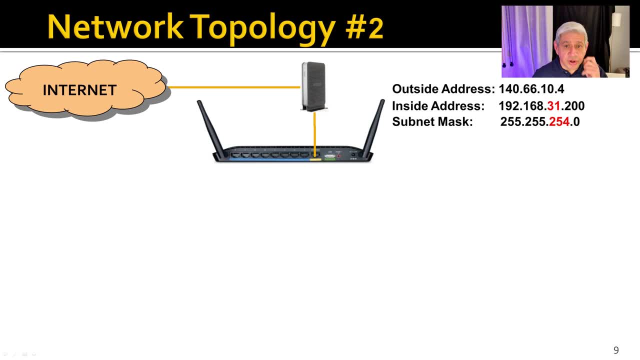 things that I've changed from network topology number one example that I showed earlier. So it changed. So 254 is a new number. The same thing here. Well, the two devices that are the laptops that are pulling from DHCP. It's very likely. There's no guarantee that those addresses will. 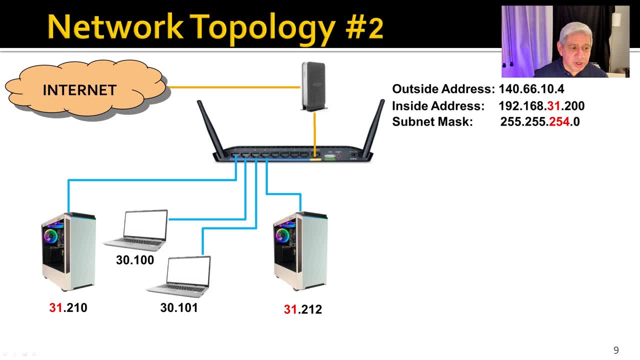 be assigned. I'm just making a guess that, since these two laptops are DHCP, those are addresses they could get, because that's within the range of DHCP addresses. However, the two servers that I have here, the two workstations- excuse me, they are going to be at 31.210 and 31.212.. Now how? 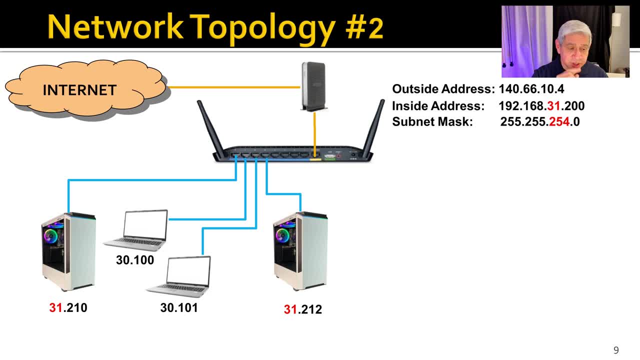 do. I know that because I'm going to set those addresses in those devices. They're not going to use DHCP to get their addresses. They're outside the range as well for the DHCP, And so I hardcode those in. Let's look at the other devices that I showed earlier. Well, now, just by pure this could. 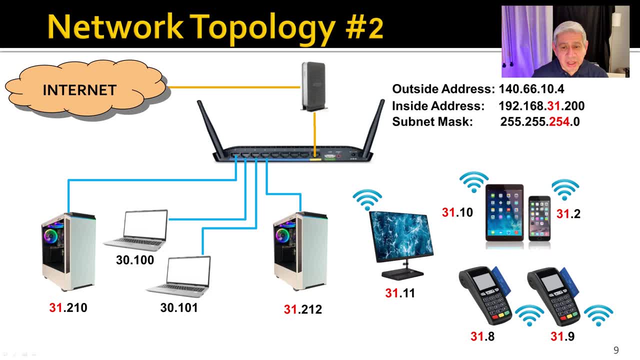 happen, There's no guarantee They could be down in the 30 area as well. I put them all at the 31 because the DHCP address range has now extended into that 31 part of the overall address range. Now let's take a look at a common network topology based. 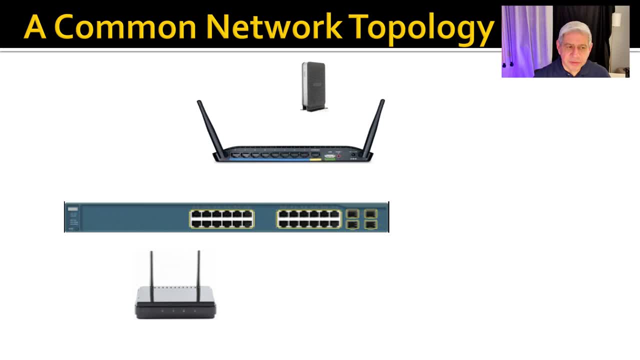 upon this, and this is going to be very close to what my network looks like. You have the internet, you have a modem, you have a router. they're, in that order, connected. then I have a switch, a main switch, with 28 ports. on it, Of course, the 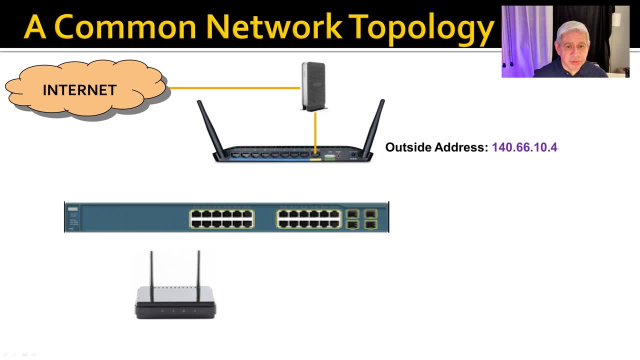 router is going to have the same address. as I said earlier, the outside address is going to be assigned by the ISP. the inside address is going to be assigned by me, hard coded as 31.200.. The router is then going to be connected to one of 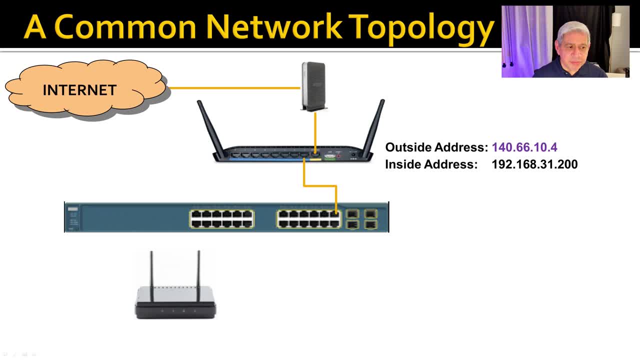 the ports on the switch. It's basically going to allow me to have that many more wired connections within my home office, because I have a lot of wired connections here. 24 sometimes doesn't even make it. I also have a smaller router Now I showed one here that is also wireless. It doesn't have to be. 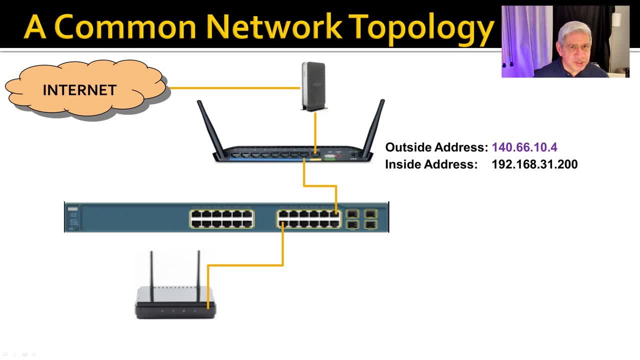 wireless. it could just be like the one that I put in for real, which is the ZYCEL one, which has an additional 12 ports on it, but I have a 10 gig connection going between my switch and my studio so that I have local connections within my studio Address. wise. 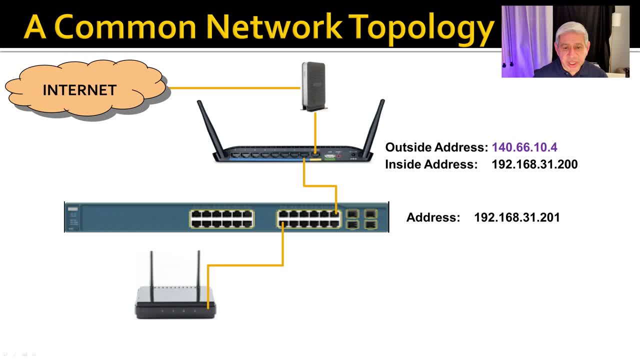 this switch has is manageable, so it's going to be given the address- again- static- of 201, and this small switch here in my studio is given the address of .202.. So this is just an example of how they all would would be in terms of the. 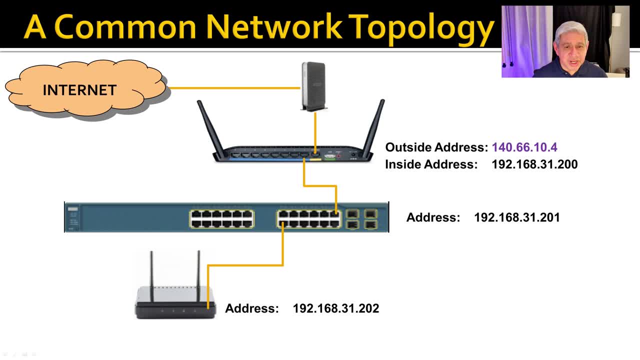 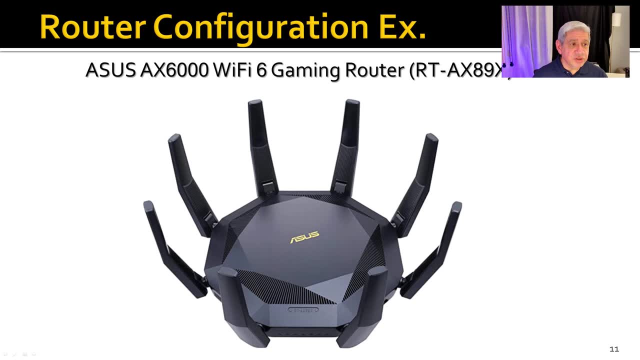 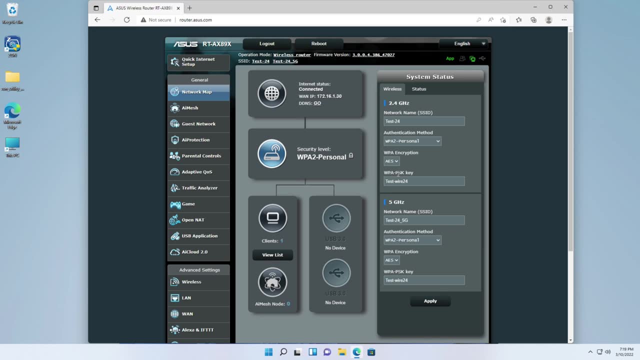 within the device range right, The routers and switch area that I defined earlier in that table. Now let's go ahead and let's take a look at the configuration of the actual router, the Asus AX89X. What I've done is I've reinitialized my new Asus RT-AX89X router, and these are the 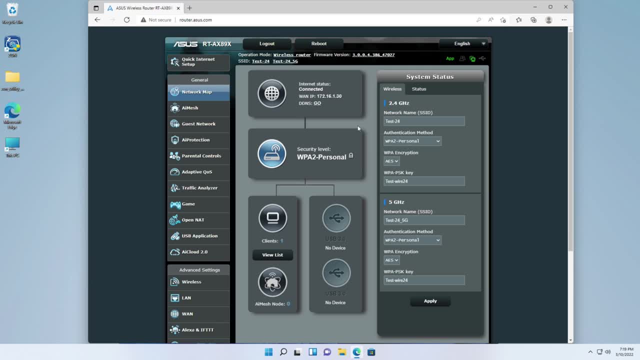 addresses that it came default with out of the box, except for the WAN IP address. That's an address that it pulled from my local network because this device now thinks my local network is the ISP, as I showed in my earlier video. I also defined, however, the network SSID names for wireless, both 2.4 and 5. 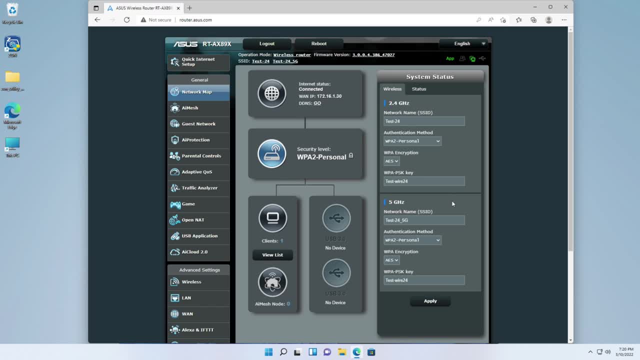 gigahertz, and I've set up the admin name and the password for admin to this. So those are the only things that I've changed. Everything else was automatically selected by the router in its default configuration, which I will now change. Let's take a look at the client list first. This is the DHCP. I have one PC. 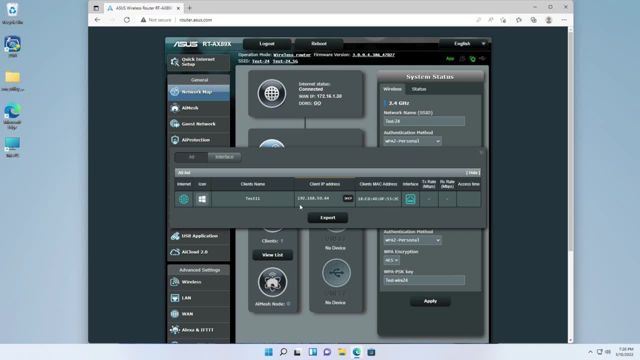 connected to it, which has the name test 11, and it assigned the address of 168.50.64.. That was an automatic assignment because that PC is set up to get its address using DHCP. It does show that the interface is wired. Now let's. 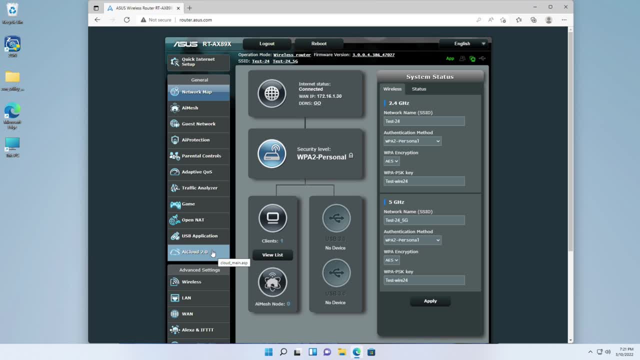 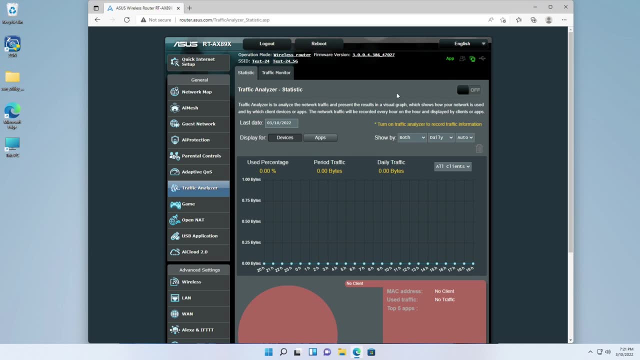 take a look at some configuration of this and we might change a few things. First of all, I suggest you go into traffic analyzer and make sure that that's turned on By default. if you look here, traffic analyzer is off. It doesn't use that much resources and it comes in very, very handy. So if we click on this, 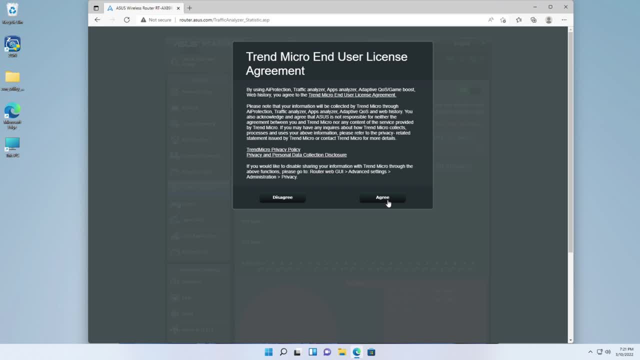 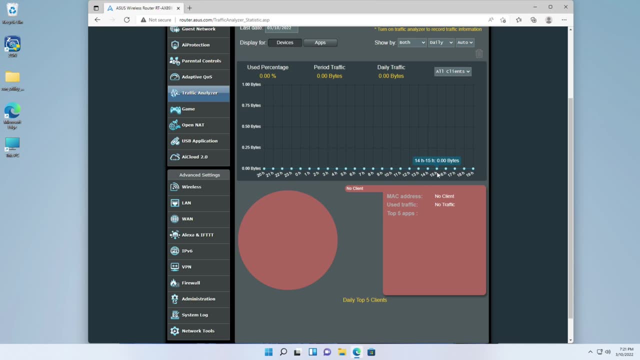 it turns it on. I have to agree to what it's going to do. That's fine, I'll agree, and it's now set up. Now, going forward, I will have a history of the actual traffic that's going through here, hour by hour, by 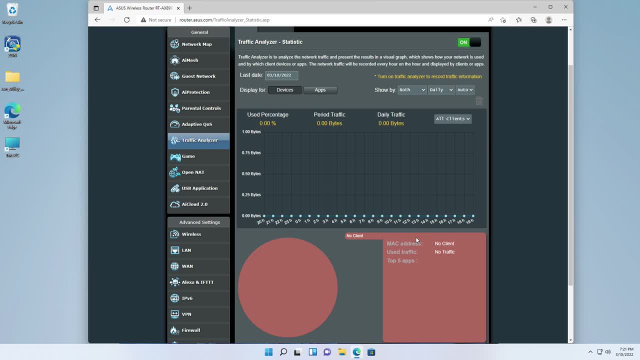 device that actually is connected to the router And you know, we'll see what it looks like toward the end and see if we pick up now some of this. I then want to go ahead and open up the the area called the open NAT. So in open NAT I 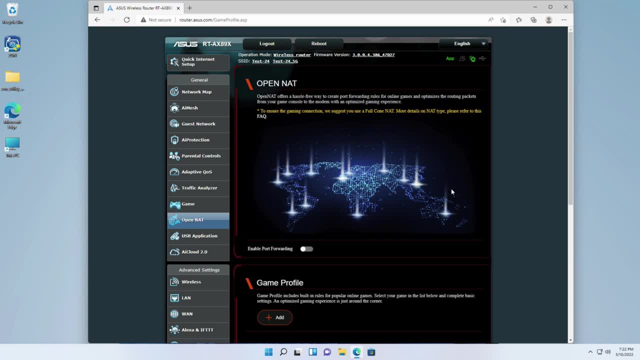 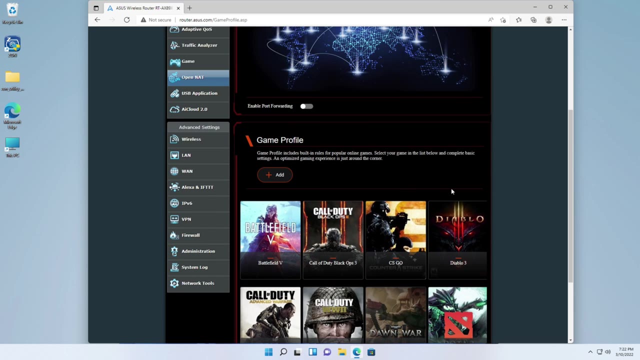 want to show you something. This actually shows the network address translation. as I mentioned earlier in the first part of this video, where the internal address is 172 addresses, It converted to something that looks like my ISP address, In this case here a 172 address range. But look at, this particular router has It knows. 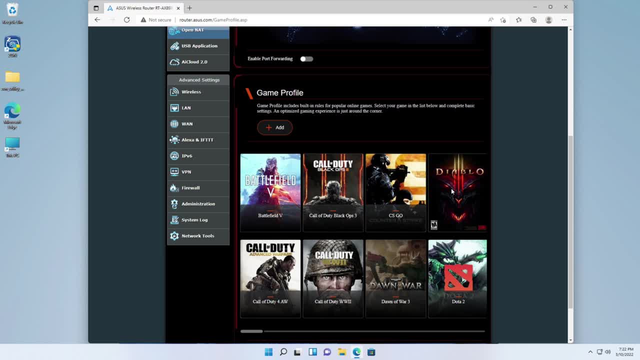 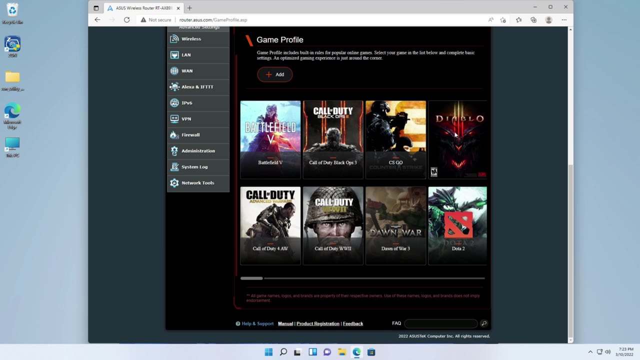 that it has to get certain ports passed through. It actually creates pass throughs for certain ports, depending on games. This is a gaming router and it has these games already connected to it and it knows what it has to set up for these games to function properly. These games will work very well because the changes 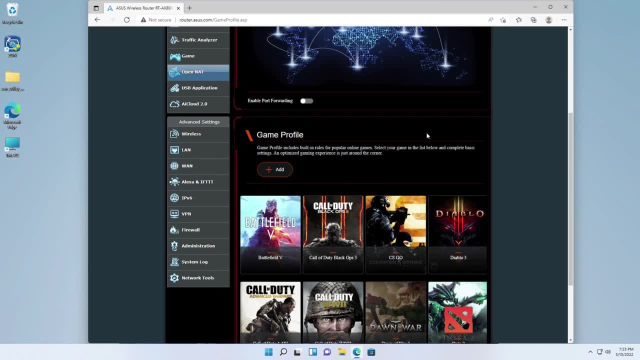 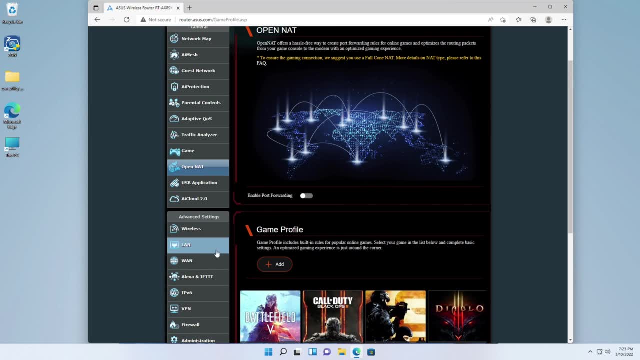 needed to the router. pass throughs are will be set properly, and you can add new ones to it as well. I just wanted to show that as something that's a nice feature of this router. if you're into gaming Now, the next big one which we can spend most of our time is in the LAN tab down here. 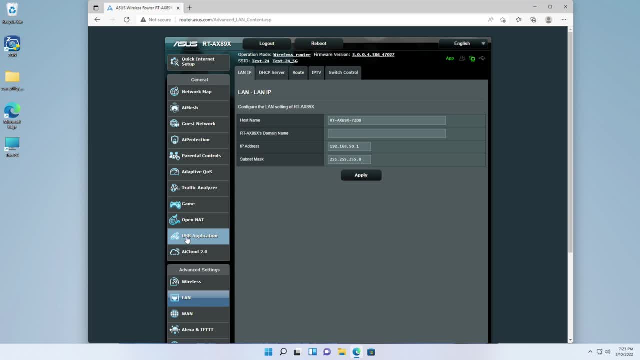 So, if we open up the LAN tab, the first thing that we will see here is a host name. Now, this is the default host name. You can change it to whatever you want, though All you have to do is highlight it and overwrite it. So let me change it. to DR-Router1, just in case I get a router 2.. But I also want to change the IP address. I don't want this address. Remember what I designed on my particular configuration. I want this address range to be 192.168.. That's fine. 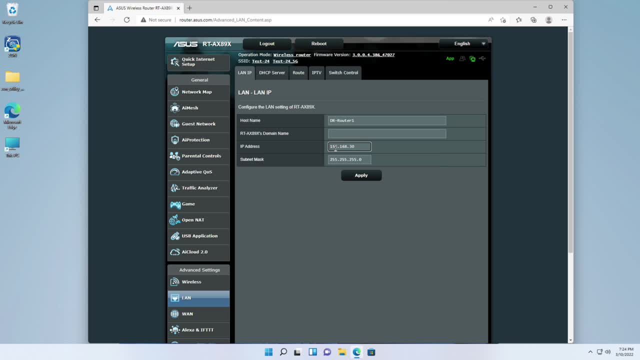 but I want to change it to 30. That's the network address that I want And the IP address is asking for. here is the actual IP address I want to assign to the router itself, Which is a Device. and, as you recall from my example, what did I? 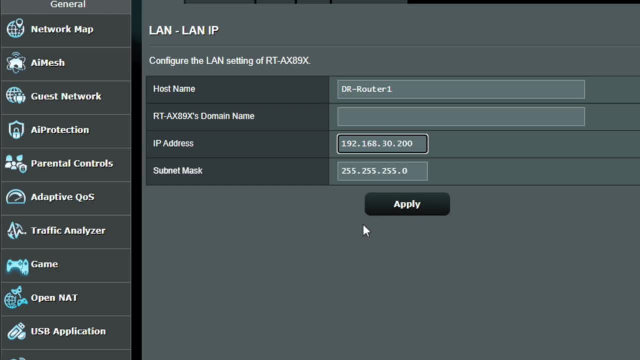 assign that device to Device 200. But I'm going to make it so that we are a net mask of 254, not 255, because I want to get the 510 addresses, So I'll change it to 4.. And those: 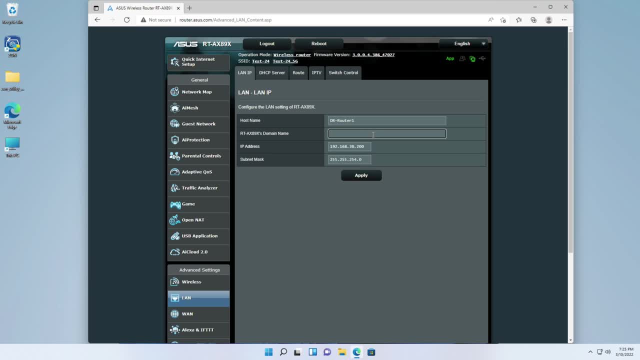 are the changes I want to make to this particular part of the LAN tab. The router will automatically know that I am setting up a 512 address range And since I gave it the mask of 254, it will know that 30 has to be included in that. It's a little bit of a trick, but it's based upon those bits. 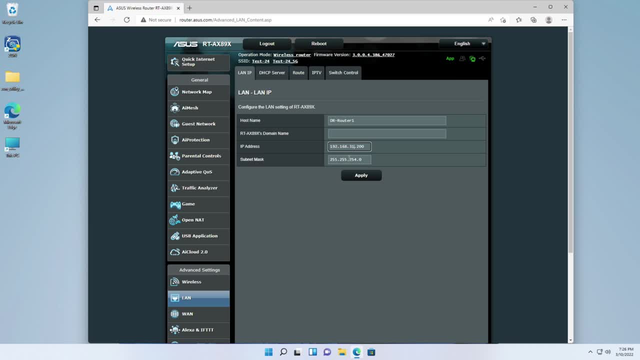 that we broke down earlier. It knows that the .31, .200, when I have a 254 mask- has to be in a range that starts at .30, .0.. So let's see what happens. when I hit Apply, It's given me a warning. 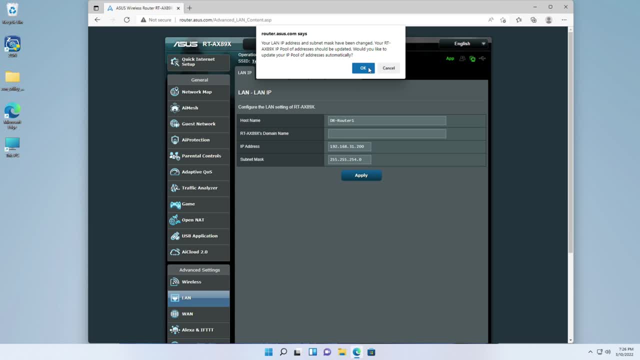 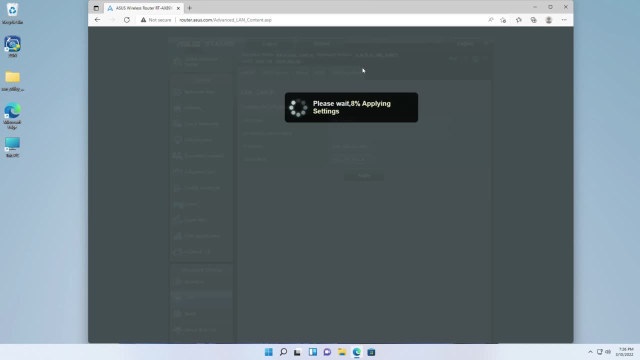 that it may move my router around and I may have to re-log in and I may have trouble finding it, But we'll find it because we know what the address is. Click OK, and now we have to wait. It takes a few seconds to go through and apply these changes. It's reconfiguring. 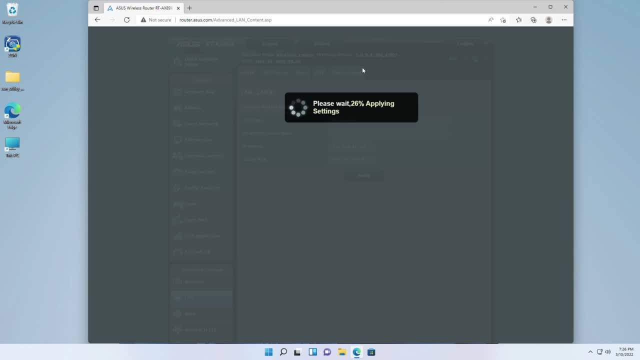 internal configuration files of the actual router itself, And then we'll see what the result is at the end. It's telling me that the router is now at 192.168.31.200.. So I'm going to hit Apply And it's giving me a warning that it may move my router around. 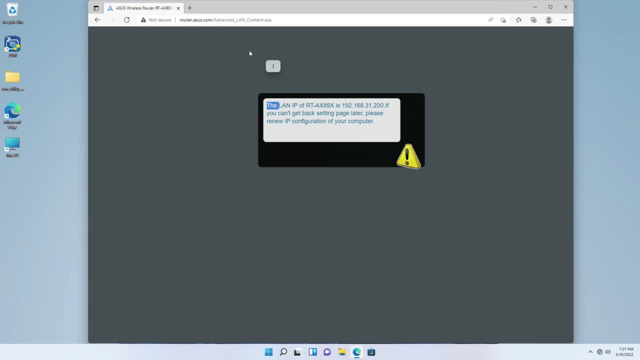 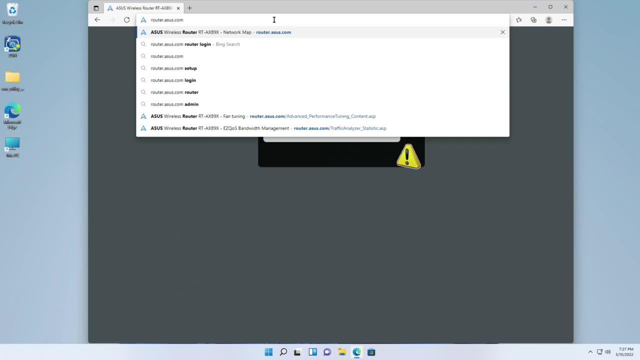 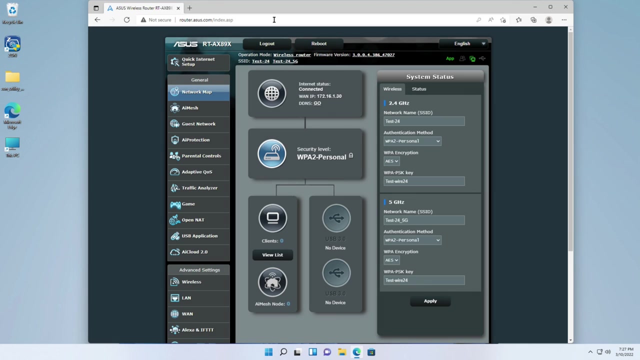 if I go ahead and click on this, it may find it, Or I could just come back up here and go back to this routerasuscom- That's a name given that it will automatically be able to find it. And there we are. I'll have to re-log in, of course, And I've signed in Now. a lot has changed, You don't? 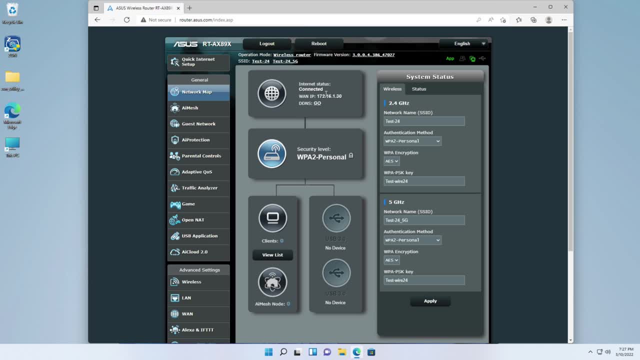 see it at first, because the IP address that's given by the ISP stays the same, But almost everything else has changed in terms of addressing. Let me start by looking at the client list. We should have one client out there. It may take a few seconds for it to identify it, But let's see. 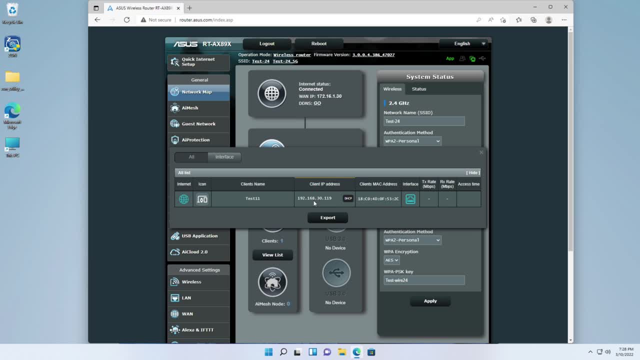 what address it assigned to that client. Now it's at 192.168.30.119.. It picked a totally different address for the same system because it has a different address range to deal with. now, If you looked at the MAC address, that did not change because that's hard-coded onto the network adapter. 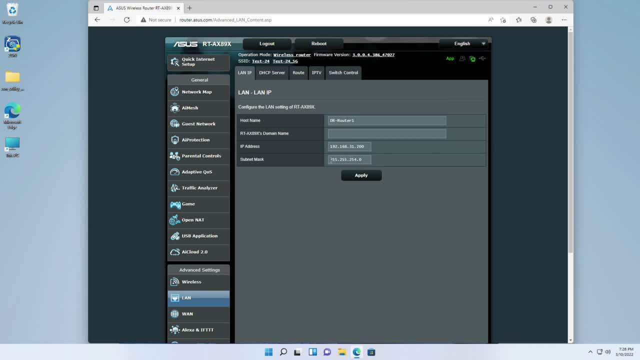 that's built into that PC. If I take a look at the LAN, what do we have here? That 168.31.200 is my particular IP for this router And the net mass is exactly what I wanted. So if I can take a look, 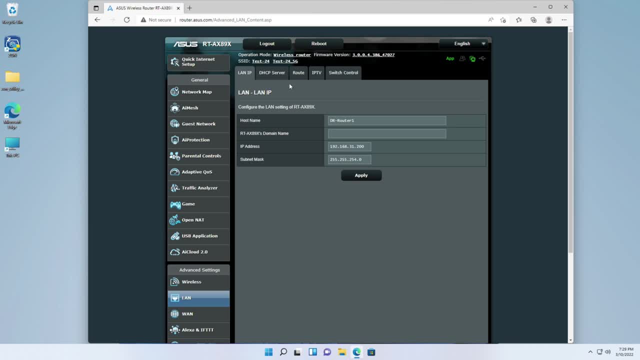 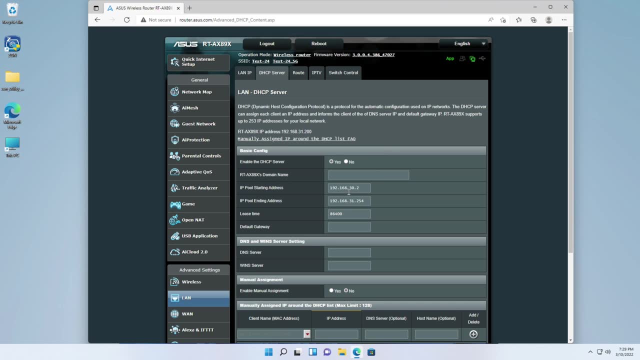 at the DHCP server. Now, I did not look at that before intentionally. We saw one of the addresses that it assigned, But let's see what it has there now. It has a starting address of 192.168.30.2,. 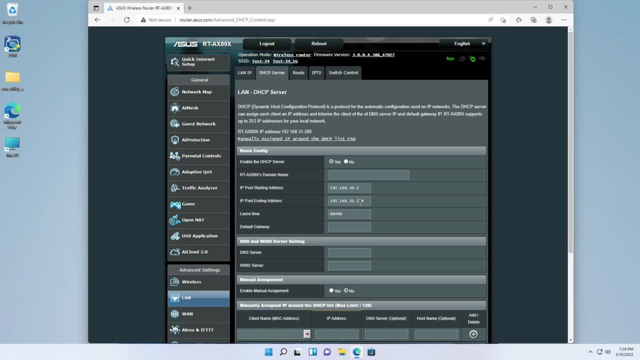 which is good. That's where I want it to start, But look what it did. It went all the way to the end: .31.254.. It basically only excluded the .1, because that's what it meant to do, So I'm going. 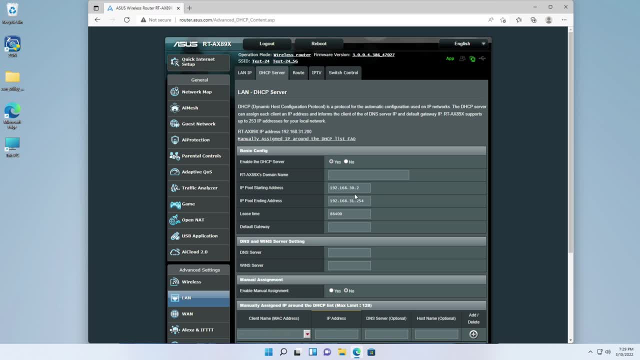 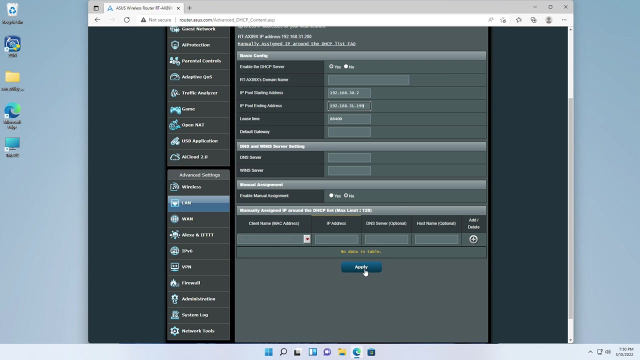 to fix that. So the address range that I want does start at .30.2.. However, it ends at .31.199.. Because I have all those reserved addresses starting at 200 to the end address that's available to me of .254.. Let me go ahead and apply this. See if it makes me log in again. 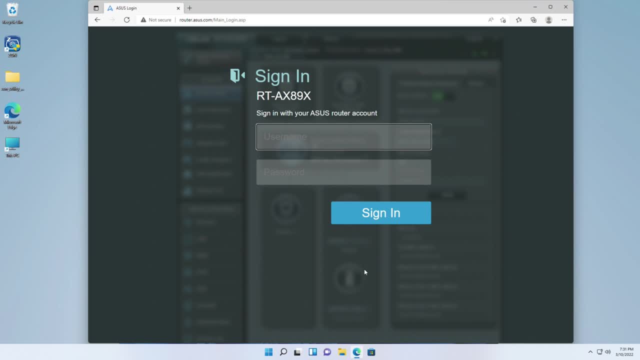 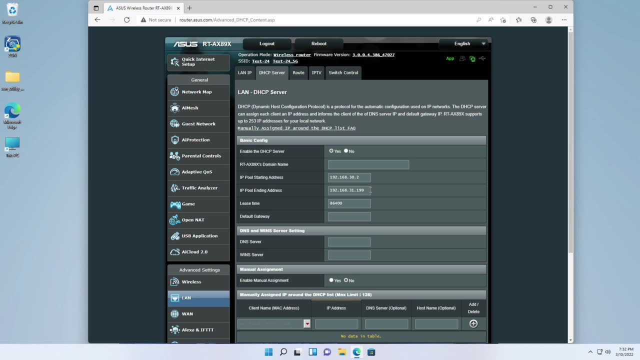 And of course it makes me log in again. I wasn't 100% sure, but there it is. Let me log in Now. it shows the new pool. It starts at 30.2 and it ends at 31.199.. And, as I showed in the table, 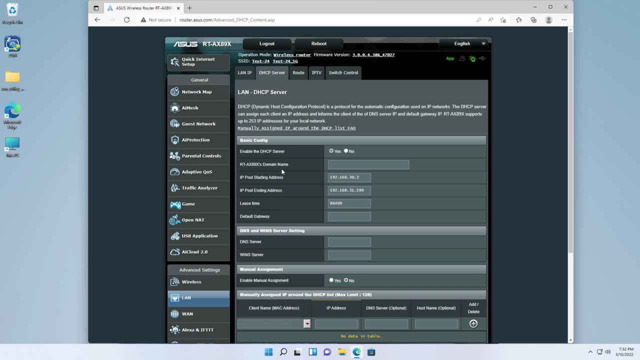 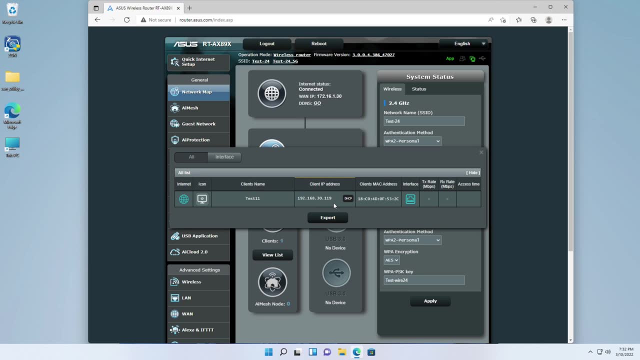 shown, it has 453 different addresses. If we go back to our network map in the front and we take a look at the one client that I have connected here, it happens to be the same address. It didn't see a need to have to change that one, So it's still 30.119.. If that address had been, 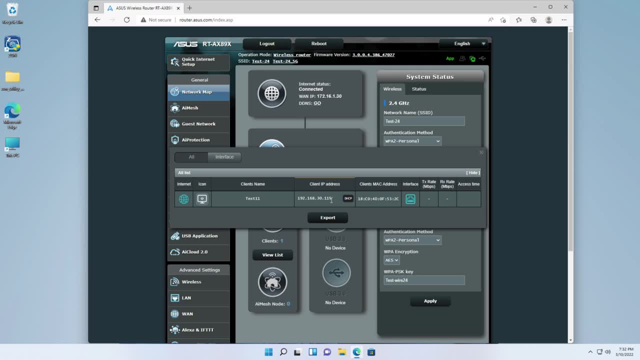 outside of the DHCP range, then it would have had to reassign it so that the PC itself would have gotten a new IP address, a new DHCP IP address. But it wasn't needed in this case. Now let's look at a couple of other things in here. Let's go back to the 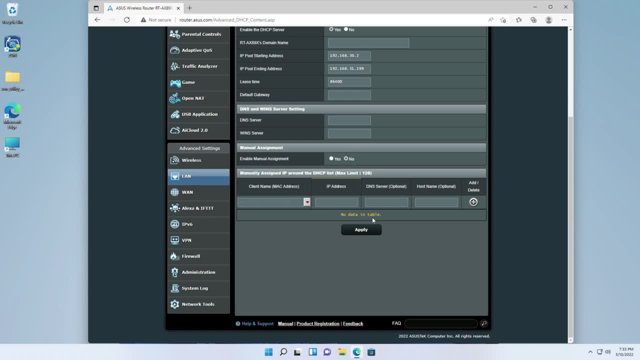 DHCP server under LAN DHCP server and let's take a look at something called enable manual assignments. This is a special case. right now it's off. Whichever one looks dark in the center is what's been selected. so the no is set. 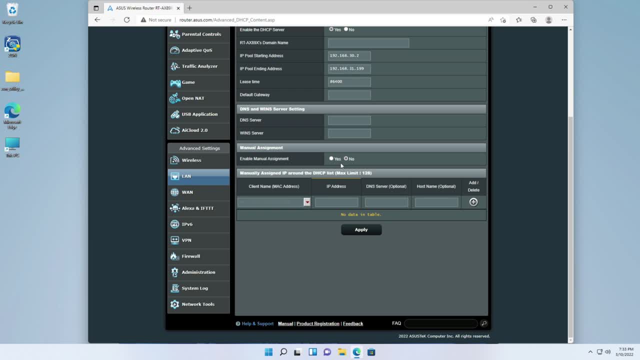 Let's say I wanted to assign a fixed address within my DHCP address. Well, I can do that. I could have left that thing to go all the way to .254, and then I would have had to enter every one of my devices that is hard coded into this table. 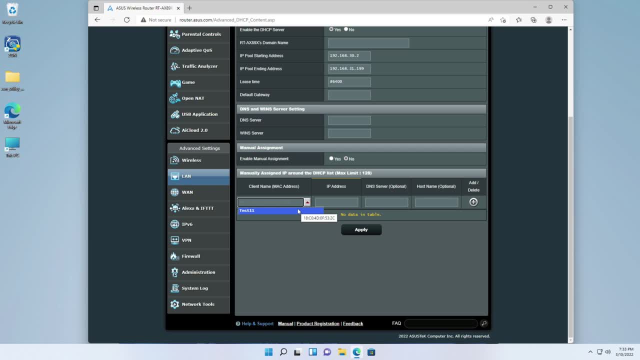 You get to pick the device. it actually sees the test 11 as the only device you can choose from and I can assign an IP address to it And I can also change its host name to something else. And if I wanted to change its DNS server, 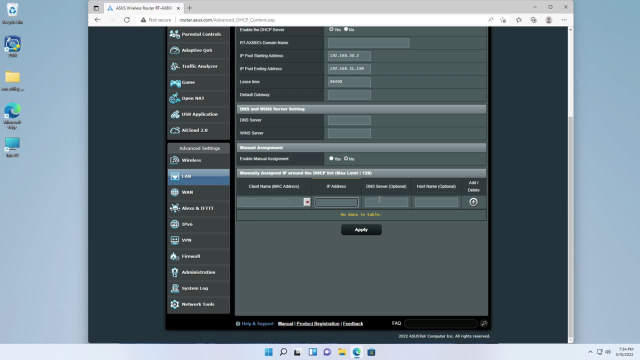 domain naming server. I could do that. That's not recommended at all- And then I could add another one, and another one, and another one. It's a very manual, drawn out process and if I did that I would hit apply. 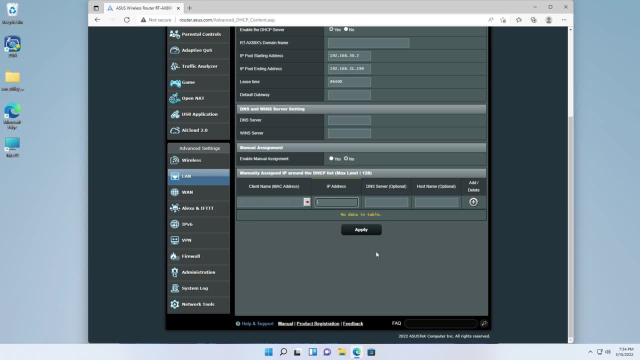 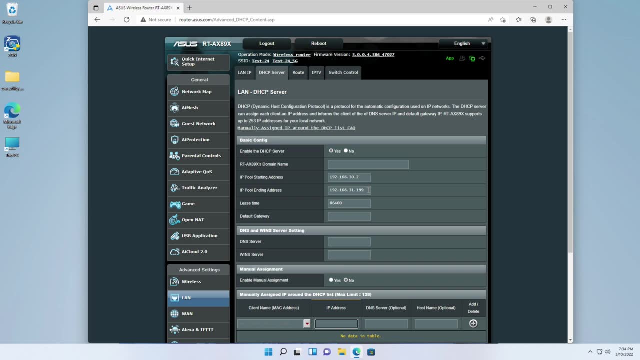 and it would then exclude those from the assignment of the DHCP. Those would be skipped, any ones that are in that table. I did it differently. I stopped the range early at 199, and then I, through documentation and the actual process I will use: I will assign the addresses above that myself, And the fact that the DHCP stops at 199, it will never interfere with the ones that I manually create above that address. I just can't go past 254, because that is the maximum for the net mask that I've chosen. 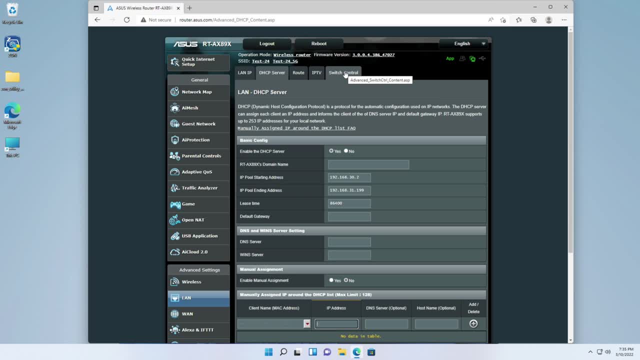 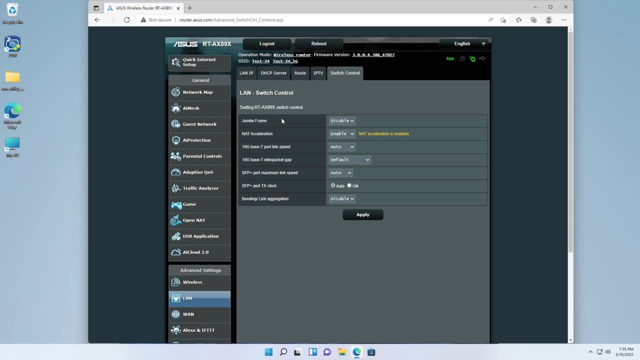 Now let's take a look at one more thing here in this LAN area, called switch control. This is important. This has the ability to control my special ports on this router. This is not covered in the manual. That's why I wanted to cover it here. 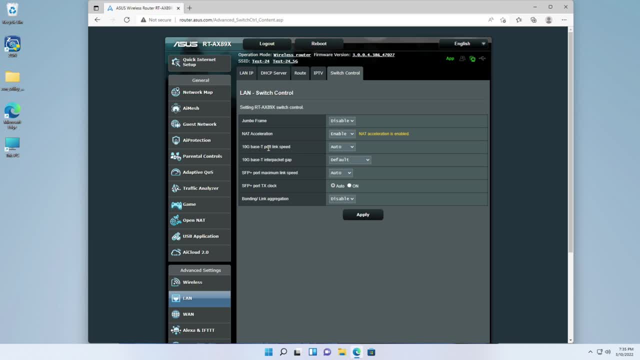 So you will see things like the 10BaseT, which is the RJ45 connector, and you have the- that's 10 gig, and we also have the 10 gig for the SFP. So there's two more ports on this particular router, right? 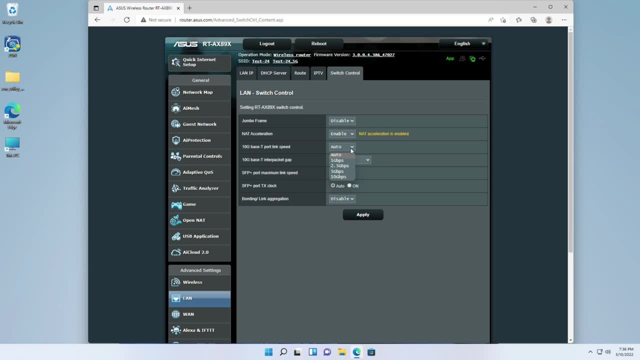 And I can assign them to special things here, For example, I can assign them to a particular speed. I can bring them all the way down to one gig if I wanted to, or I could fix them at 10.. I want to fix mine at 10,. 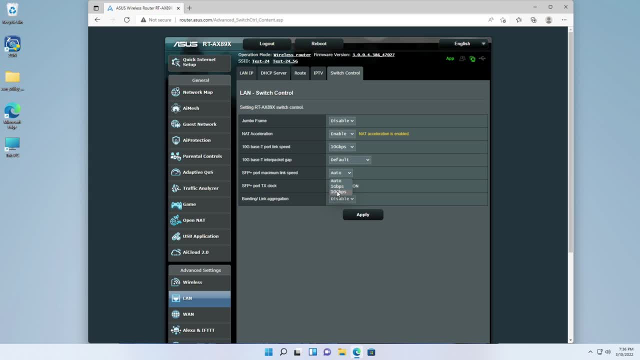 because I will be using them only at 10.. So I'm going to assign both of them And of course the SFP can only go one or 10. It can't handle the 2.5 and the five. that can be handled by the other port. 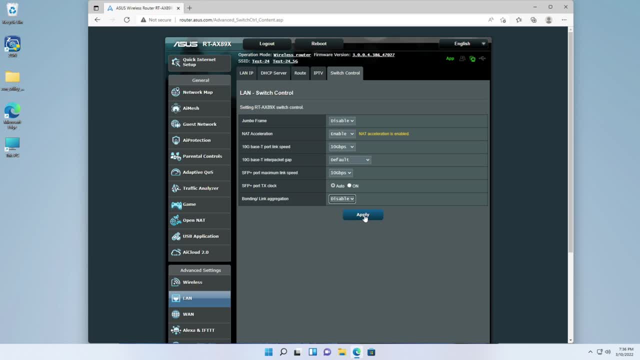 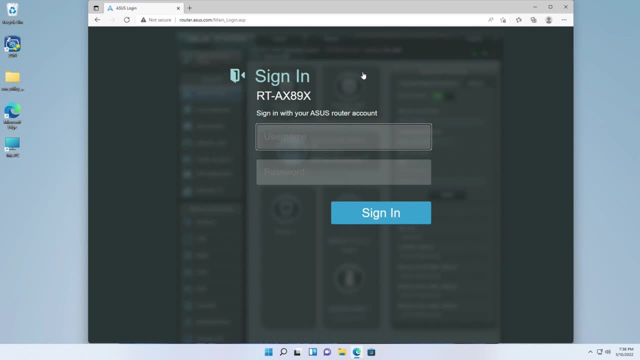 But it's the fact that these are left off. I just wanted to cover them here. I would then, of course, apply that It's probably going to log me out again. I knew it was going to log me out again because I saw it reboot.